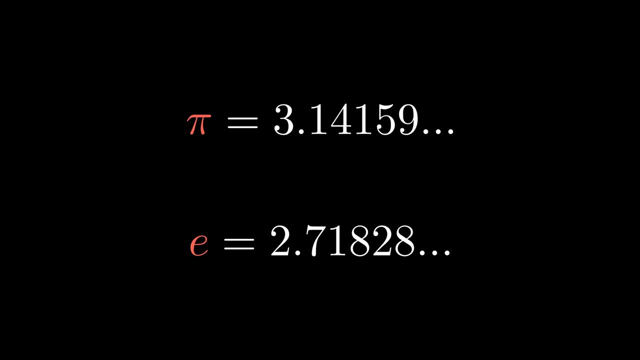 Euler's number e are reserved for special constants. you will see all over mathematics. If you see a symbol with parentheses to its right accepting an argument, you are most likely looking at a function. There are special functions such as log of x and sine of x and e to the x, but there are operators that can be done on functions. 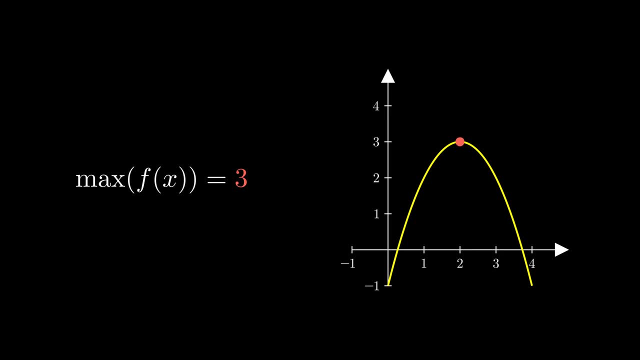 such as max, which will return the maximum output variable that can be achieved with that function, which is 3.. There is also argmax, which does the same thing, except it finds the input variables. that achieves that maximum output variable. There are minimum counterparts as well. 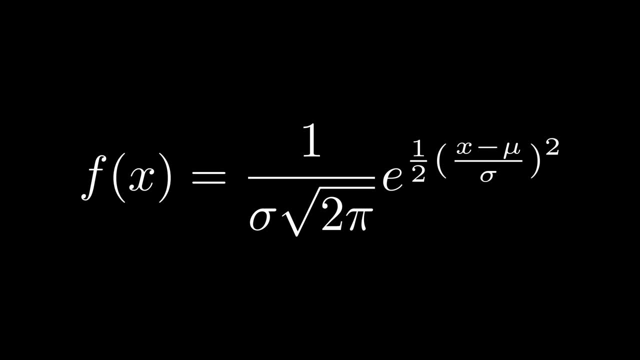 Let's take a look at one more function example: the normal distribution. As you can see, there are our two constants, pi, and Euler's number e. We saw those earlier. Mu and sigma are the mean and standard deviation respectively. They control where the bell curve is located as well as how spread out it is. 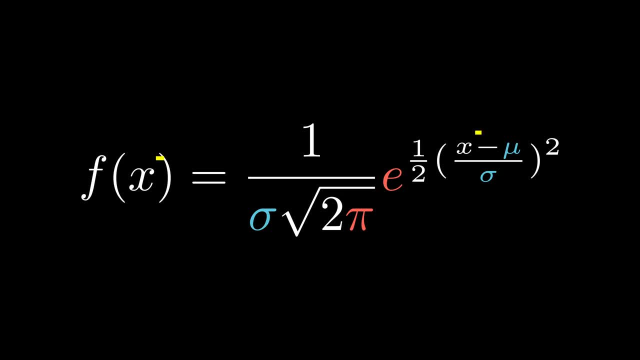 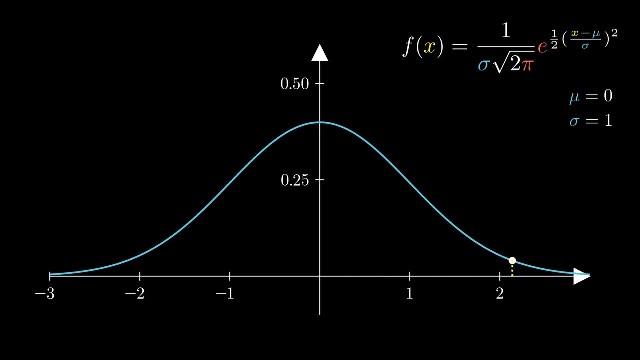 Those are calculated beforehand and are fixed. This leaves us with only one variable, x. Everything else is fixed, and then we can produce our bell curve function. So what about when you see a variable with a subscript of i? What exactly does this mean? 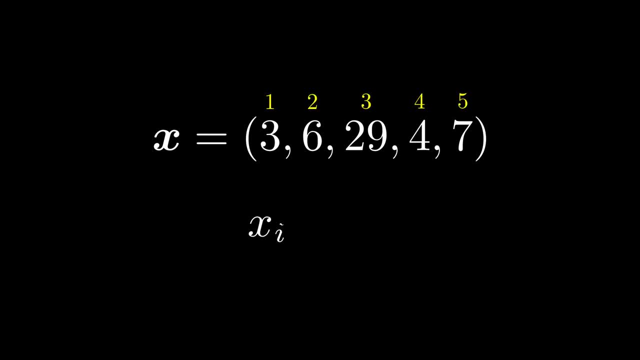 This indicates that there is a collection or vector of numbers belonging to a variable. We can access one of those elements by that index. Note carefully that traditional math notation uses one-based indexing, not zero like many programming languages. If you see an uppercase sigma, more than likely you are dealing with a summation which essentially says: add up all of. 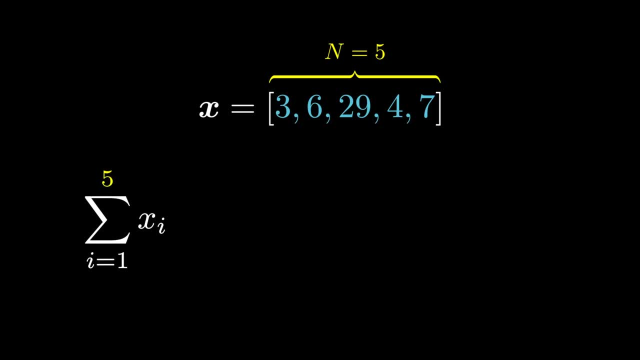 the x elements together in a given list or vector. Since there are five elements, you would read this as: 4i equals 1 through 5, add all of those x elements together, So we can see that there are four x elements. 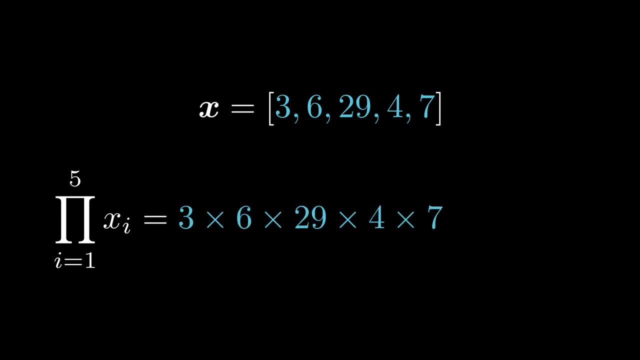 The uppercase pi is the multiplication counterpart. It multiplies all the elements in a vector or list together. You can add decorations and modifiers to a given symbol to specify a different context. For example, x-bar can specify the mean or average of all the x values. 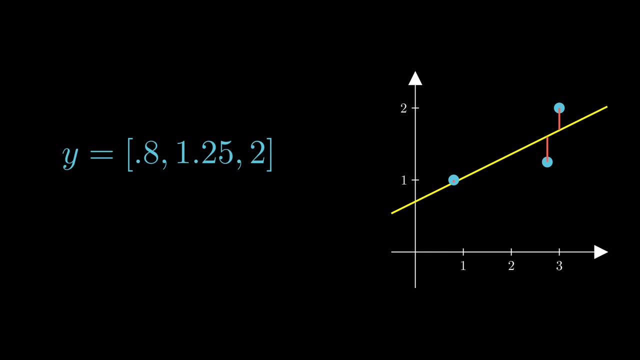 Another example of modifying a variable for a different context is when you have a variable for a particular context but if you do not have a variable, you will need to add a new variable to the variable. Another example of modifying a variable for a different context is putting a hat on the y-value.